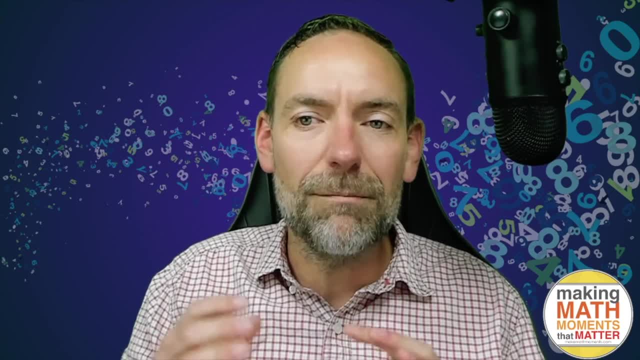 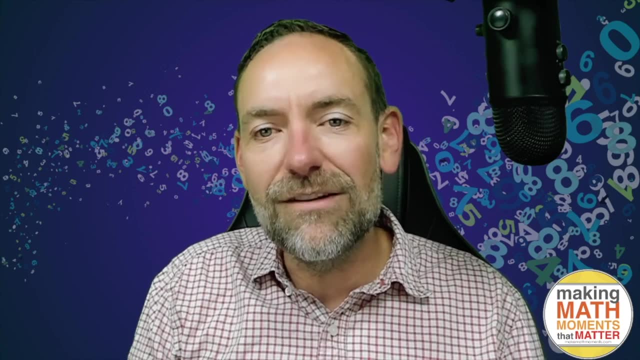 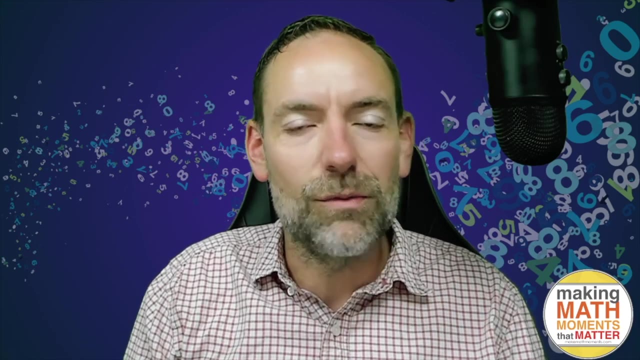 a learning, a skill. further down the developmental road is not possible until students have mastered an understanding of prior skills and concepts. Well, in today's video, we're going to show that we can begin our learning journey with an idea. In this case it's going to be ratios, rates and 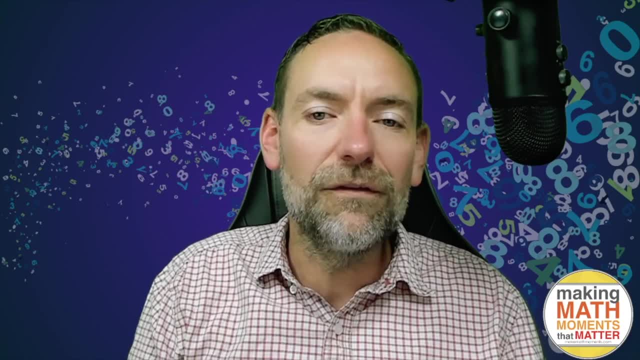 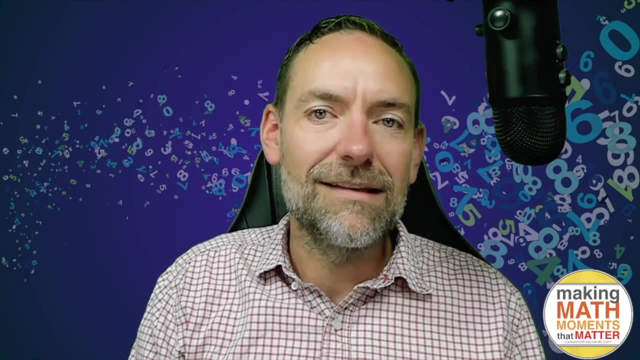 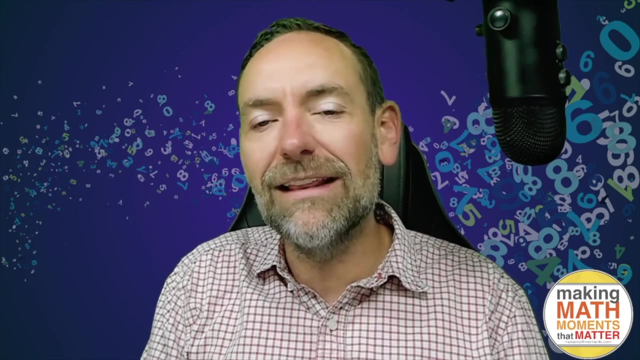 proportional relationships as a means to build our fluency and flexibility with multiplication and division, Instead of waiting for mastery in those concepts before moving on to this super important concept. So in this video, we're going to talk about how we can leverage context and mathematical models. 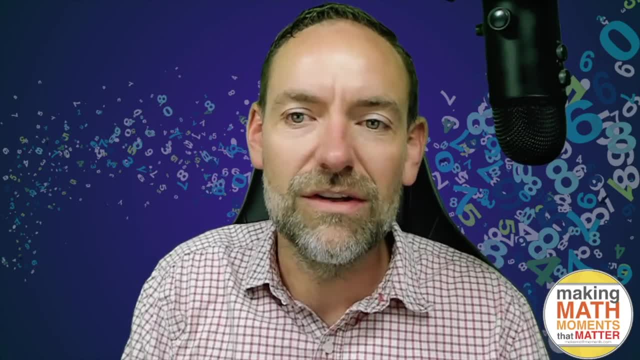 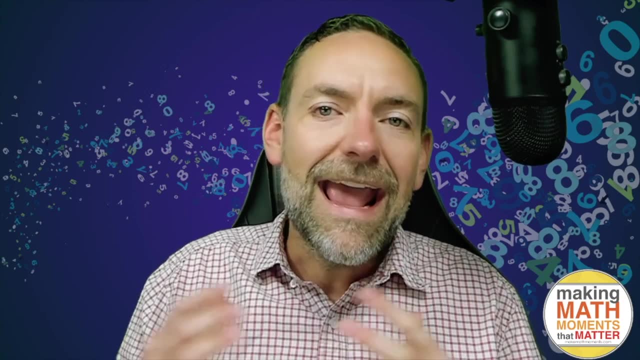 Actually, I should say we're not going to talk about it. We're going to show you how you could do that as a means to introduce ratios and rates, while building fluency and flexibility with multiplication and division. And we're also going to show you at the end of this video where you can 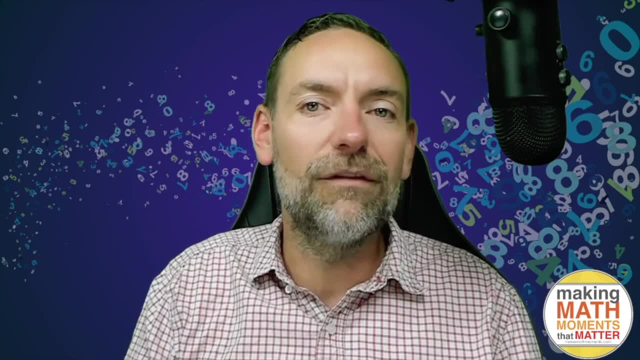 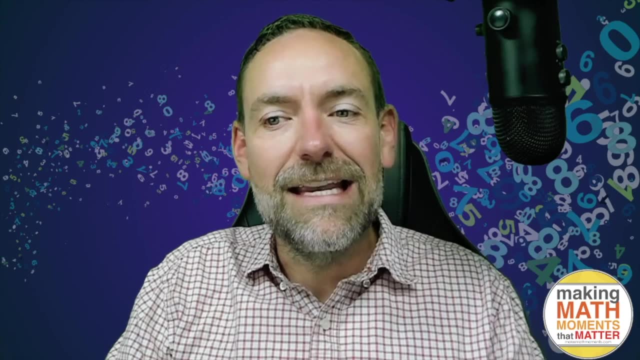 go to find the problem-based use of mathematical models. So let's get started. We're going to start off with an example of a unit called planting flowers that we are modeling in this particular video. All right, my friends, get ready, because here we go. 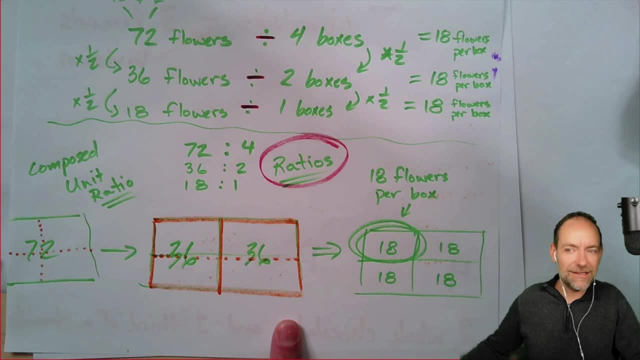 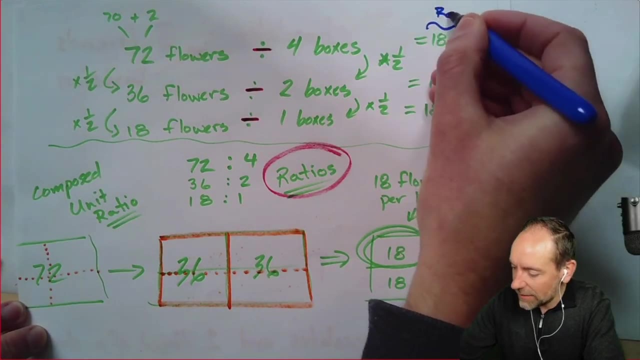 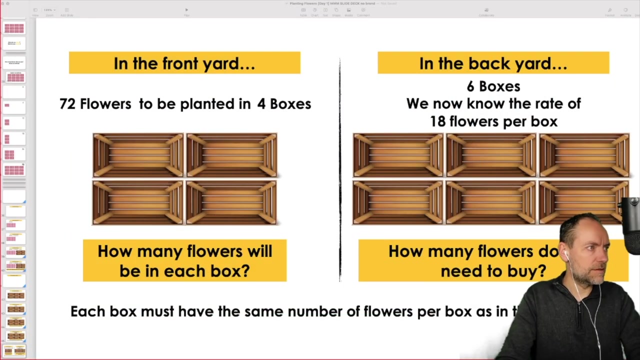 This was the actual problem, right? This was the actual problem, right here. Now you're telling me that, okay, wait, this was the rate that we had revealed. We found the rate the other day, right, Awesome, I love it. Let's do that right now. 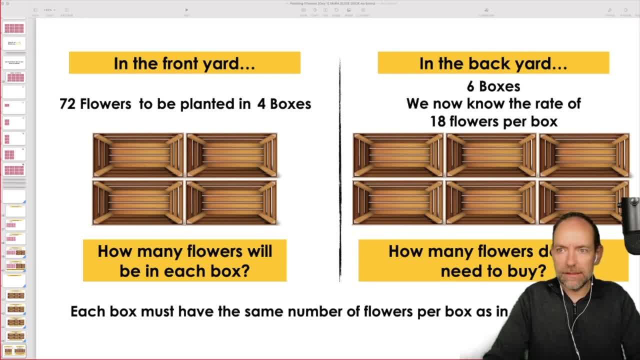 Awesome, I love it. Let's do that right now. Awesome, I love it. Let's do that right now. Alright, we'll be back in just a few minutes- a timer bars coming out for you. Alright, we'll be back in just a few minutes- a timer bars coming out for you. 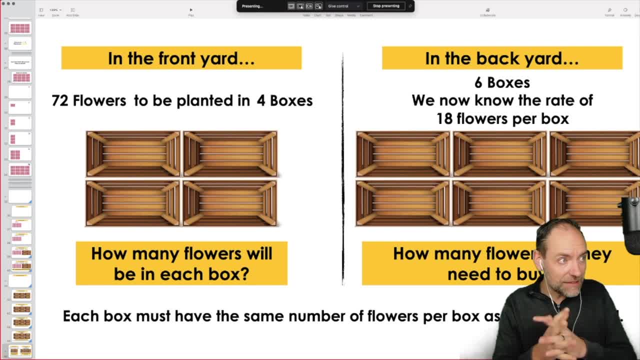 Okay, so now I do see a couple strategies. I also I also see some misconceptions that are very common. And you know, we look at this problem over here and we think about it and we go place a second, And we think about it and we go wait a second. we have 72 flowers to plant in four boxes. 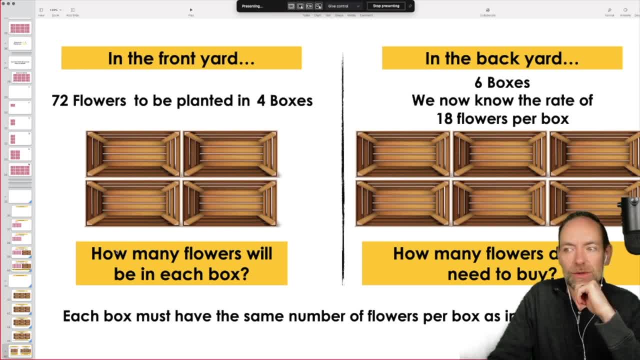 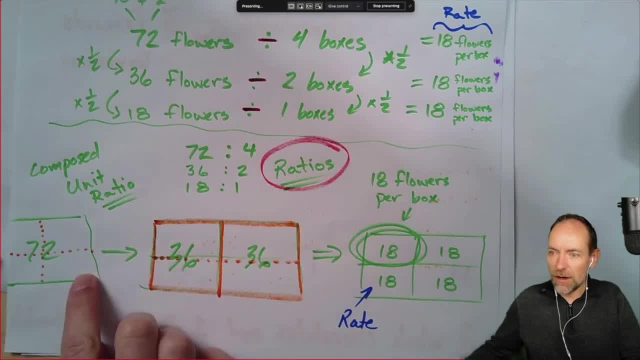 There they are. I have 72 flowers in total. There they are, I have 72 flowers in total. we kind of looked at this. we did this. you know this process of taking the 72 boxes and four. there's four boxes total. we said you know what, let's split them into two groups, two boxes each. 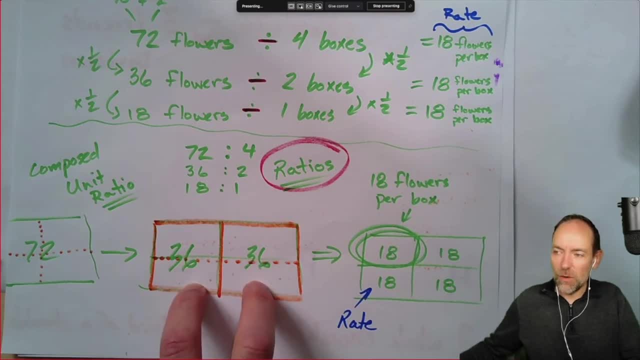 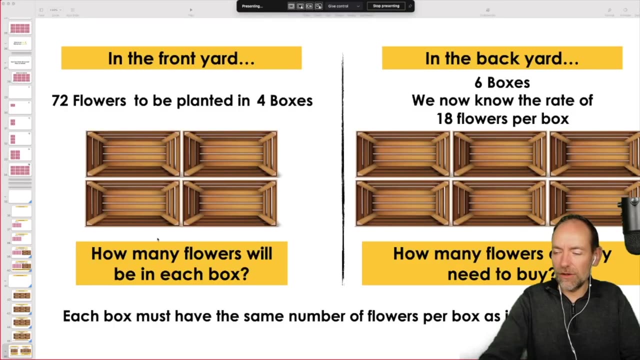 for each group. then we said: you know what that means. if we do it one more time, we're going to have four boxes and four groups of flowers, and we're good to go in this problem. here, though, we now know how many we want in each box. so i have six boxes. i need 18 flowers per box, or i need to. 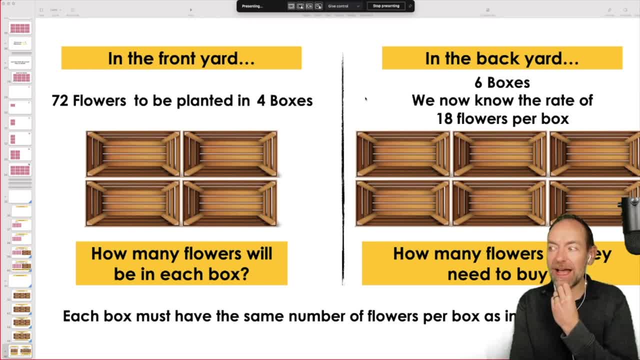 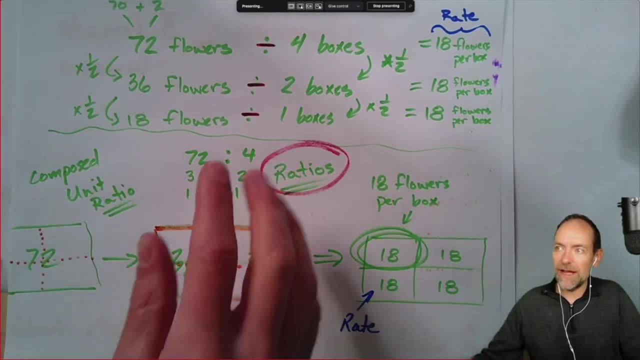 use 18 flowers per box and i want to know how many flowers in total do i need to buy? so some people may have looked at what we did and tried to just model what we did right and and i i don't know if i'm saying that, um, clearly, but like some people might have been like, well, if i just 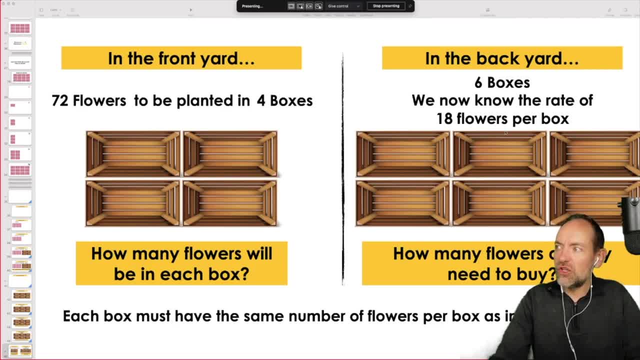 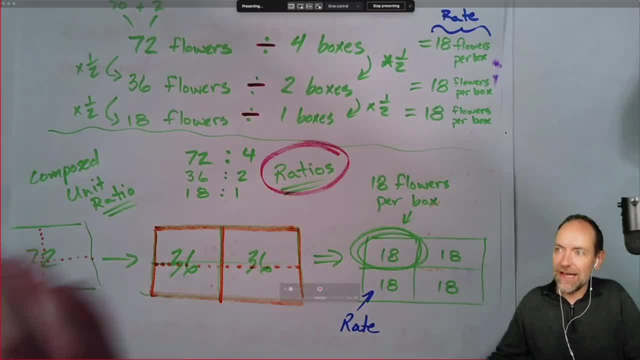 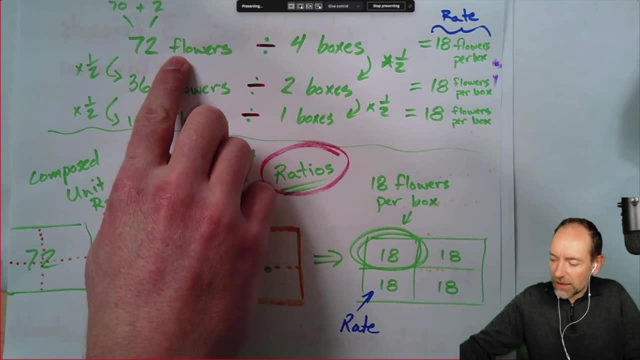 take. you know the numbers from here and i do the same thing, like some people might say. well, i see, a big number is 18 and a big number and the smaller number is six. they might go okay, 18 and six, but that's 18 flowers per box. wait, where's 18 flowers per box? that's way over here. that's the. 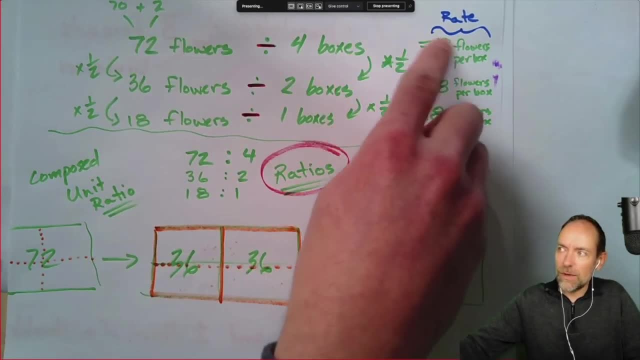 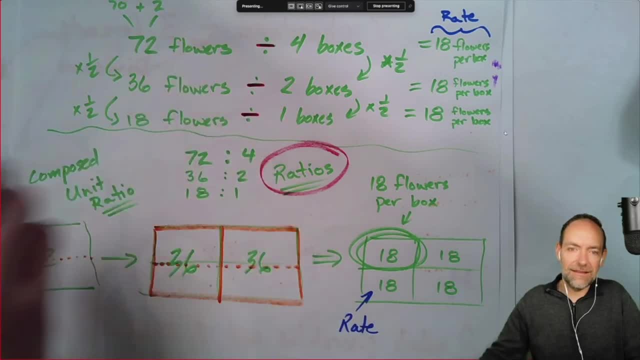 this number is now. wait a second. that is not going to um, you know that is not going to have us use that same exact strategy, although, um, although you know, again, i can see how that might happen. so for our friend that i'm going to emoji you with a surprised look, that means that you may have 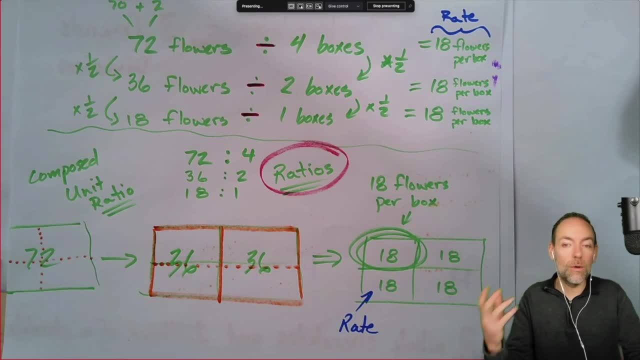 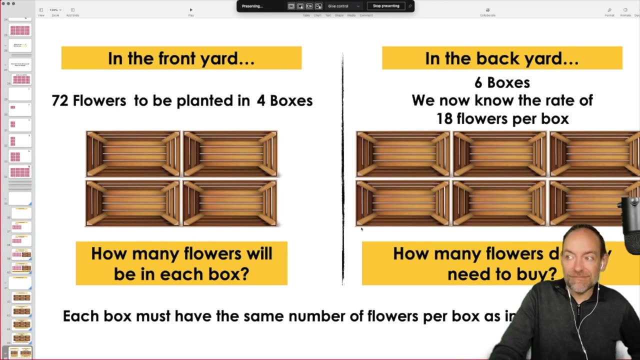 maybe misread or misinterpreted what the actual question's asking. yeah, like if i, if i was just to think about these two boxes, i mean i could, i could basically tell you like i know that if there's 18 here and there's 18 here, that i'm gonna have double 18 because i have two boxes. 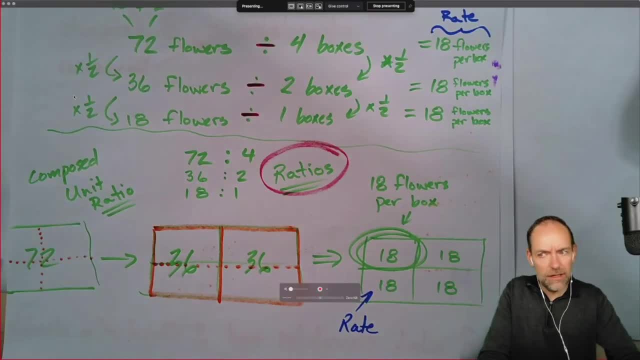 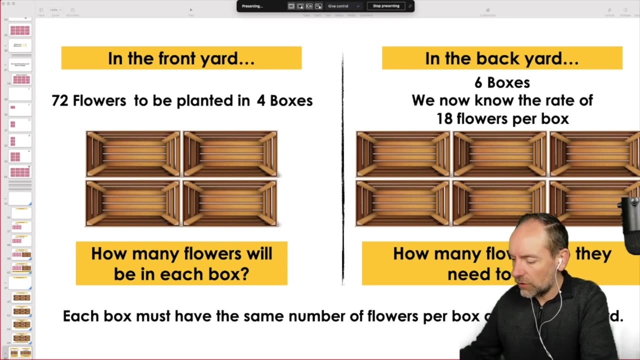 oh, interesting, i wonder if i can use a strategy like that. hmm, interesting, interesting, okay. so i'm going to pull up a nice clean sheet of paper here and basically what i think i heard you say was: like you're like, okay, well, i knew, i knew that i have six boxes. six boxes and 18 flowers per 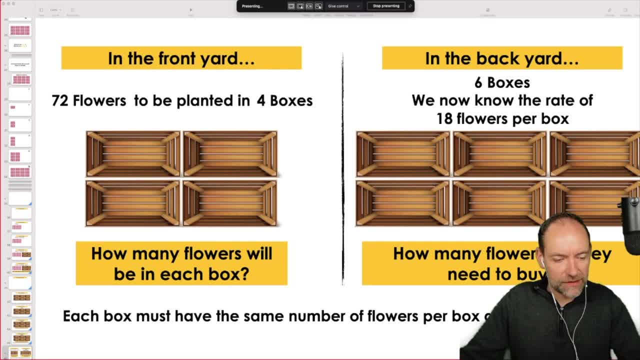 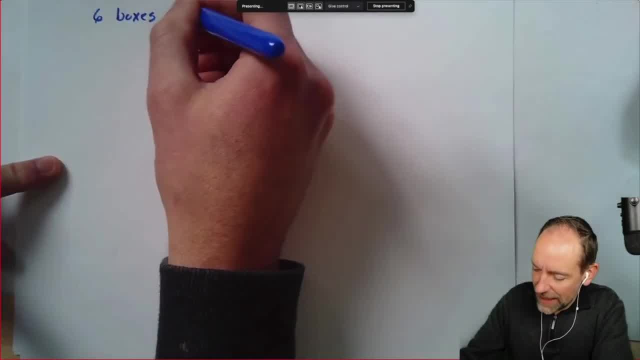 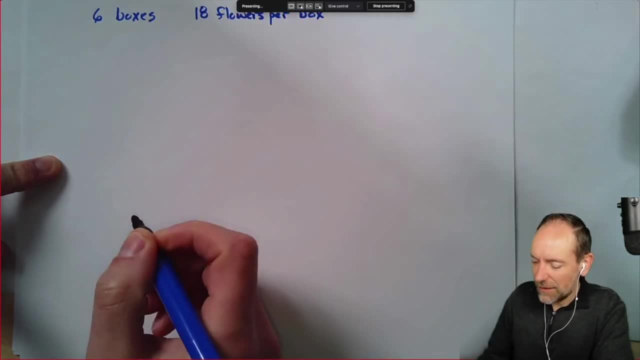 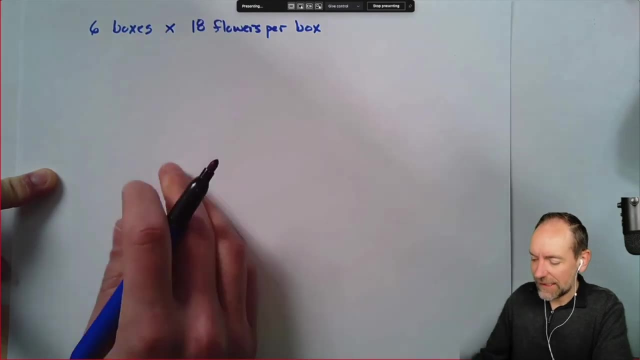 box. so it's like six is my parts or my groups. so i have six boxes and i have 18 flowers per box and we're are we dividing these two values like what are we doing multiplied? let me think about that for a second. okay, so if i have six boxes, 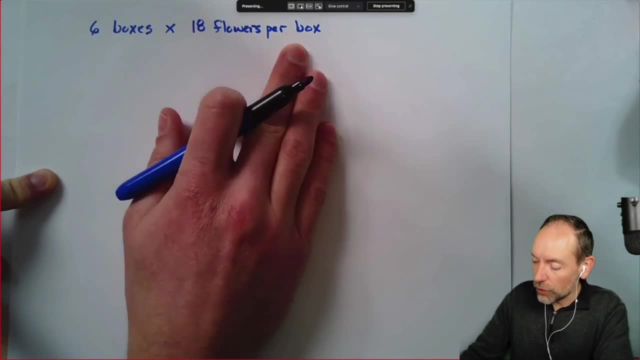 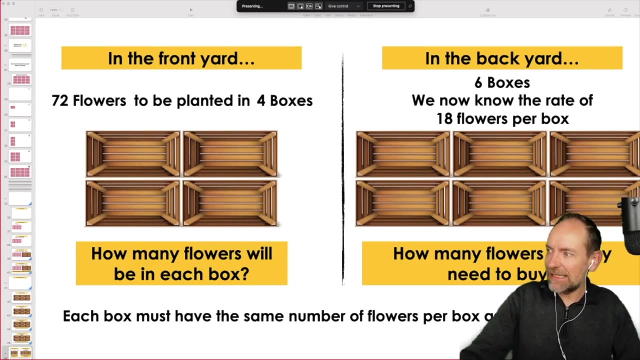 six groups of 18 per group. that kind of makes sense, right? i've got like. i've got like: yeah, it's like, if this is 18 right here, then i have like one copy, two copies, three copies, four copies, five copies, six copies or six boxes of 18 flowers per box and 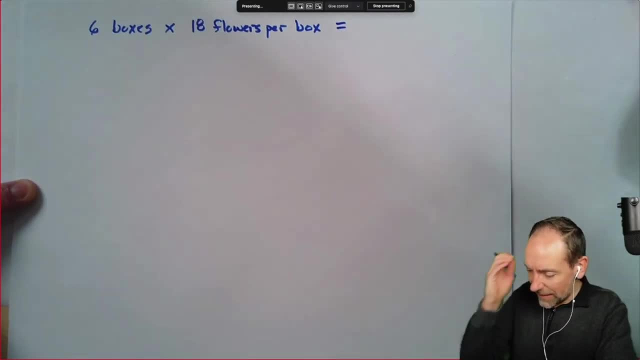 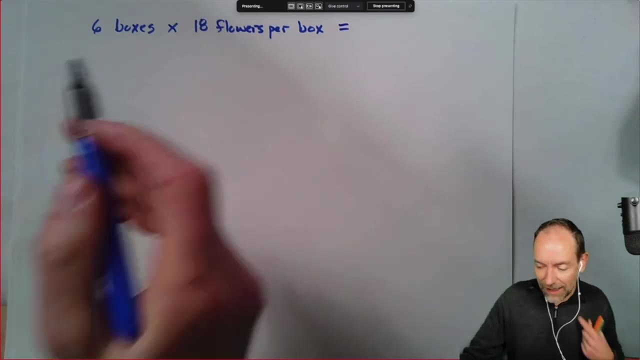 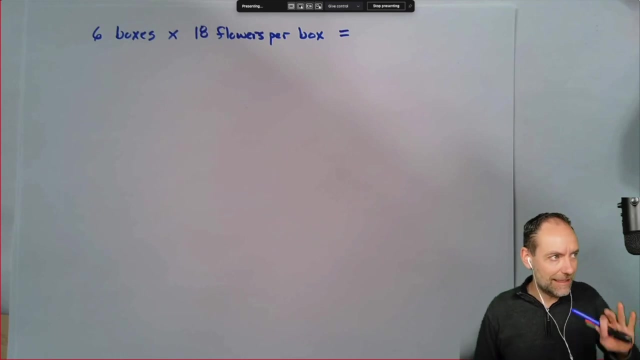 we're trying to figure out, like how much that is, and i don't know about you there, miss, but like how do you, how do you think, like did they go further? and and tell you about that, i don't know my 18 facts. uh, personally, maybe you do at home and that's cool. if you do, yeah, like keep those. 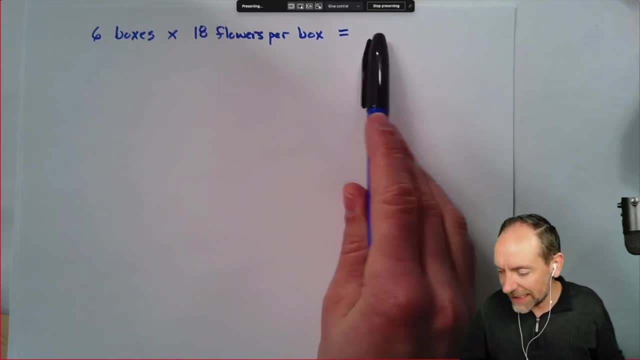 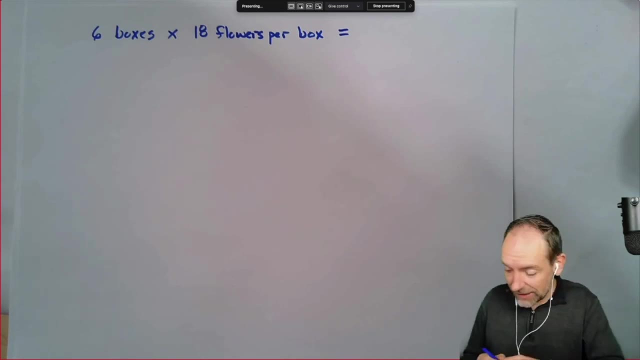 strategies coming and like one thing i'm i'm gonna not put down an answer yet, just because i'm like you know you. you say you got it right, but i don't know what your strategy is yet either. but one thing i am gonna do down at the bottom- and i wonder if this will help at all- is like i do remember the 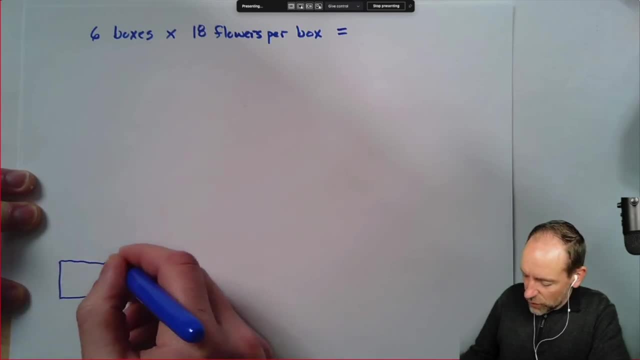 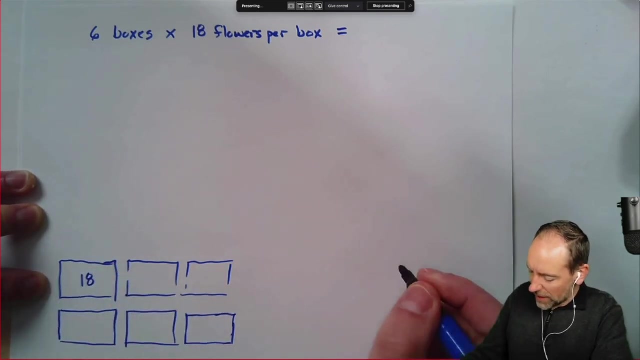 way the boxes were arranged. now, something that's really cool is that just because the boxes were arranged like this in this particular problem doesn't necessarily mean i need to keep them arranged like that, right? yeah, so like i had 18 in this one box right here, okay, that's cool. um, so i have 18. 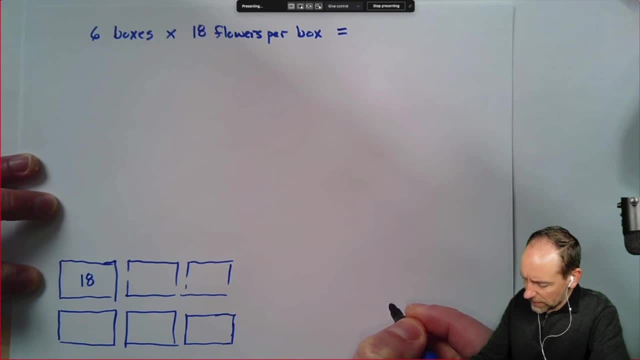 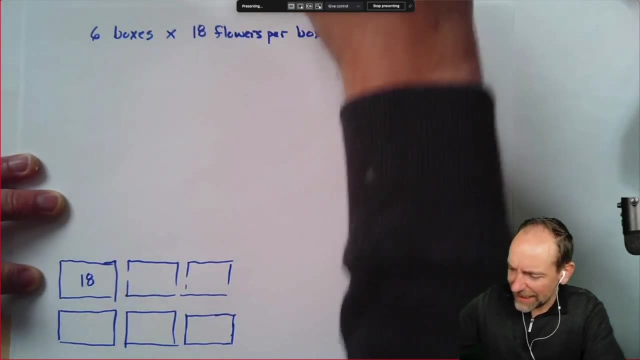 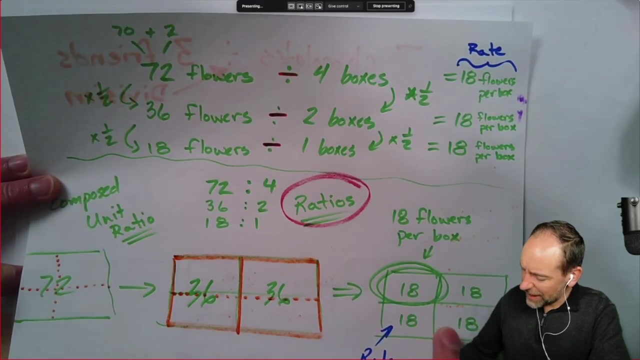 flowers per box. that's all right. um, like, how am i? i'm wondering, is there something i could do to? i'm kind of going back here and thinking like you had this strategy of having, but it's almost like. am i wrong if i say it's almost like? well, we know this. 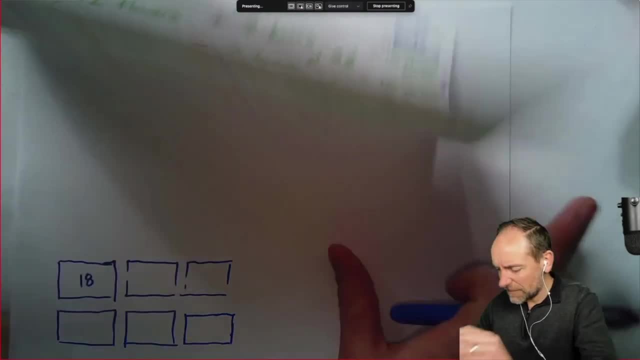 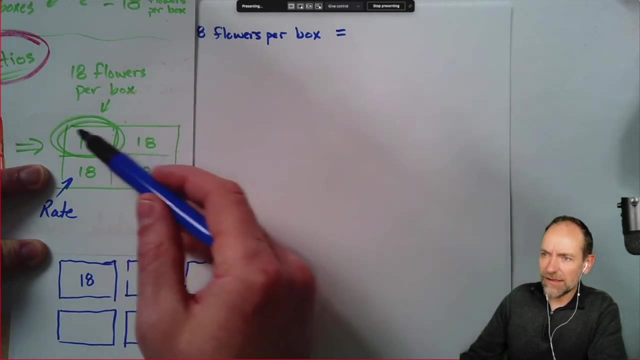 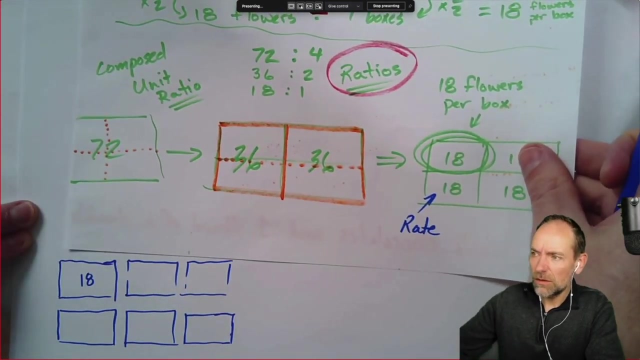 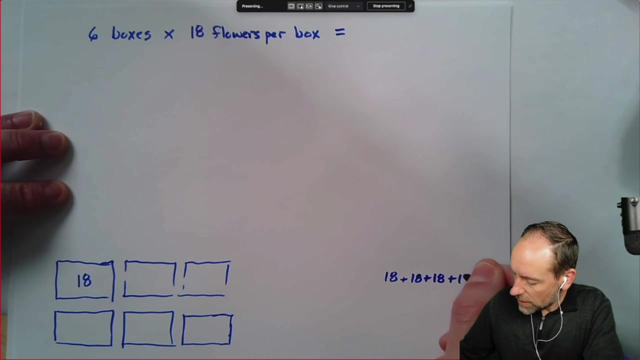 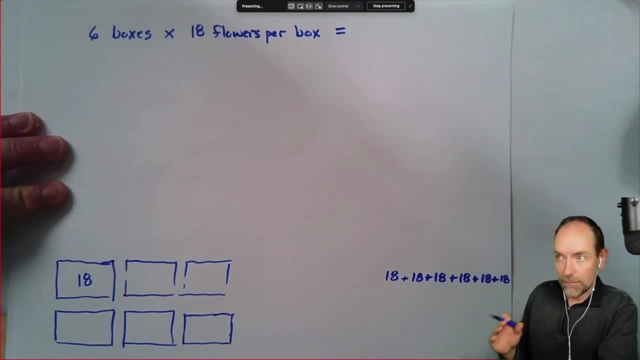 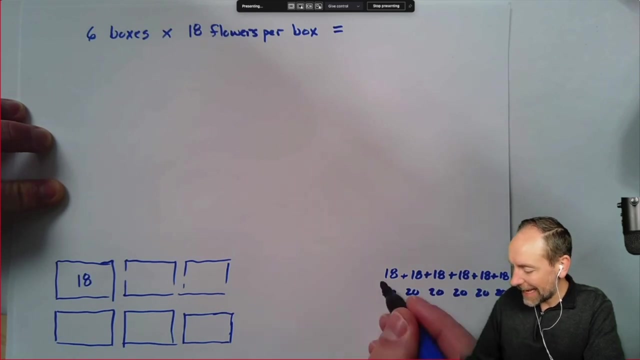 i look at that and go like that feels still hard to me, uh, personally, but it maybe it's not for for you and that's awesome if that's the case. um, something, if i was using this strategy, something i might think about doing is like: well, this feels easier to me. yeah, that's kind of my thinking, is like: if i like, add to. 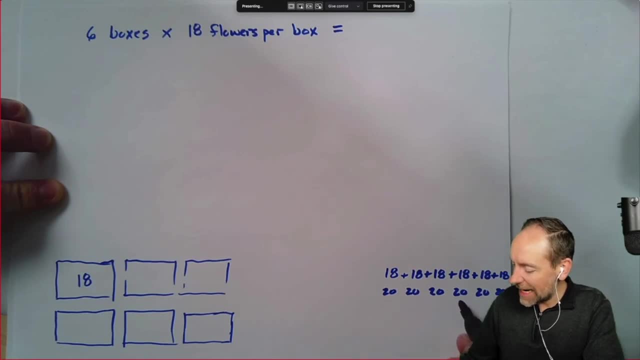 to every 18. i'm like 20, 40, 60, 80, 100, 120, but then i need to like subtract to a bunch of times. yeah, like i'm like i know this is four, i gotta take away or six. i gotta take away or wait six. 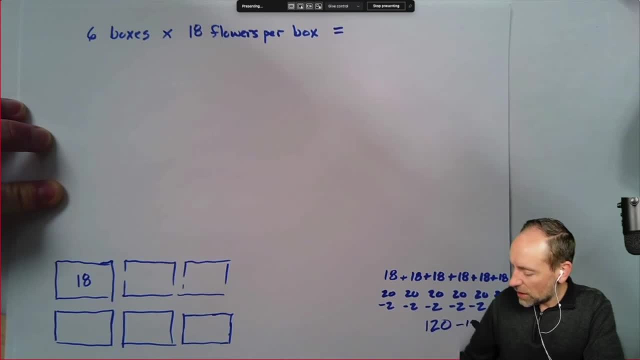 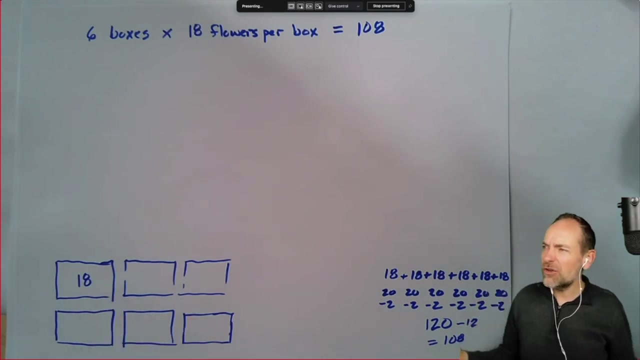 doubled is 12, so i could like go and do that and say 10, take away another two, okay, 108. so 108 feels good to me. i'm gonna put 108 here because we have three people who have said it. uh, three 108, what 108, what? what were we looking for? uh, well, if i'm 18 and we're doing that, so this is. 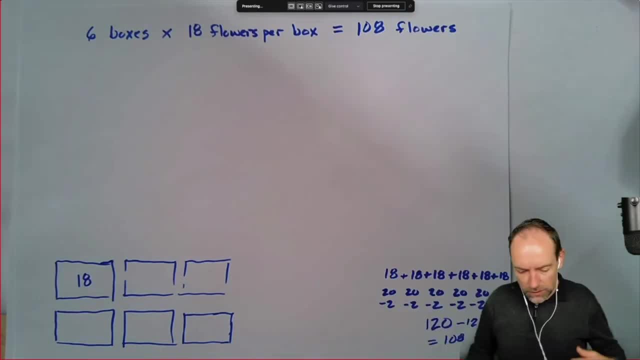 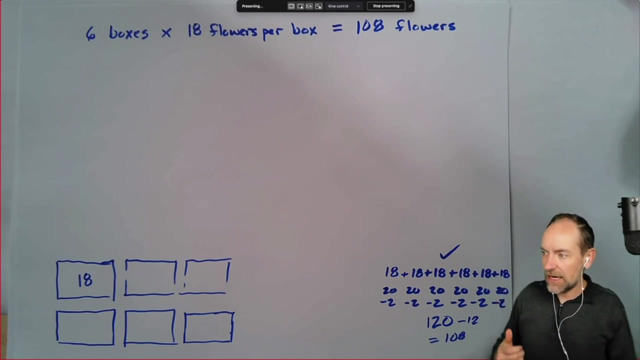 flowers. right, like this: is how many flowers in total? okay, this strategy to me super cool, like so, whoever added 18, 18, you didn't have to add it the way i did, but that to me felt easier for me, so that's why i did that strategy, but maybe you had a different. yeah, somebody may have had a better. 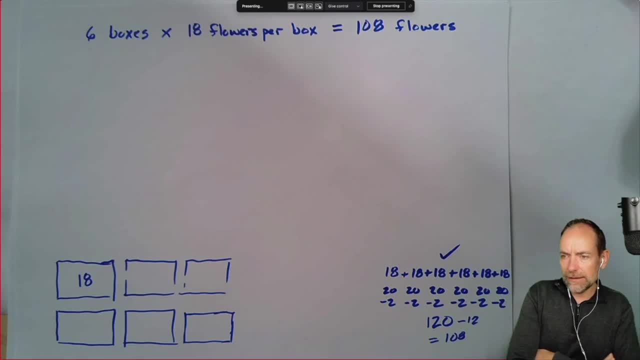 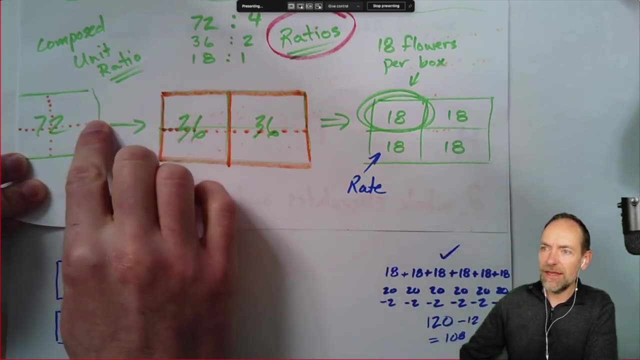 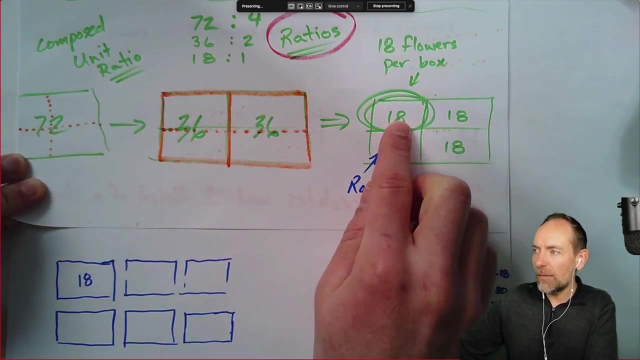 or a different strategy there. okay, now i'm wondering, like i want to come back, like miss, is it okay if we come back to this thinking for a second, because i'm curious to see if my thinking works, because, like, we had flowers and then we wanted to figure out how many per box, and now we know how many per box and i wonder if, like, we work. 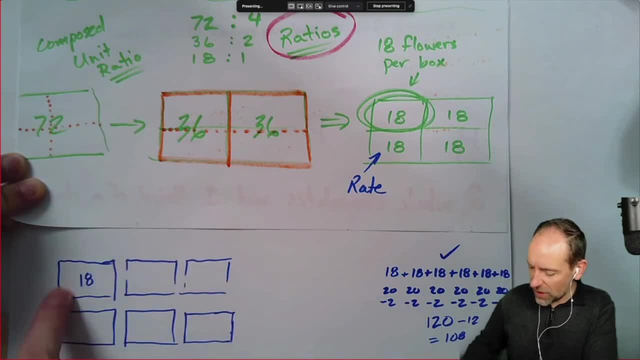 back that way. like i'm feeling confident that these are equal to 72 flowers, i'm also confident that these are equal to 72 flowers are equal to 72 flowers, but i've double counted. if i do that these are equal to 72 flowers. like i, i know a lot here. 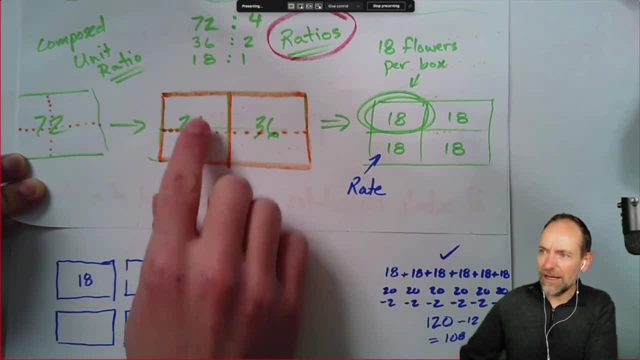 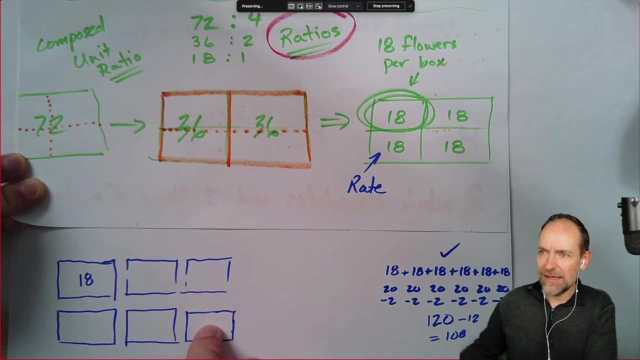 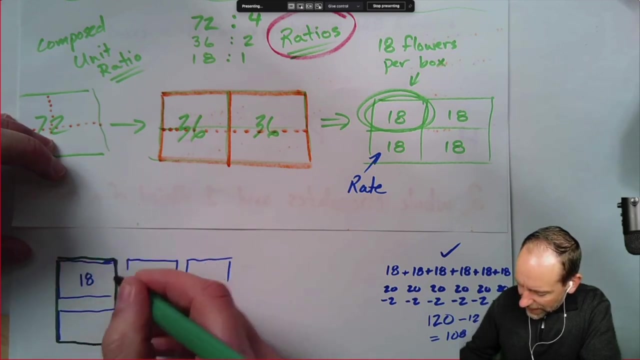 when i go over to here, i feel like two boxes is 36 flowers. so i'm seeing a lot of ways that i might be able to use this information to help me get there, like i. i'm sort of thinking like if i look, this is 36 flowers. 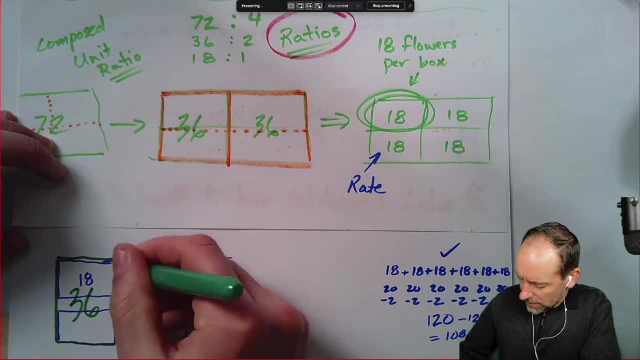 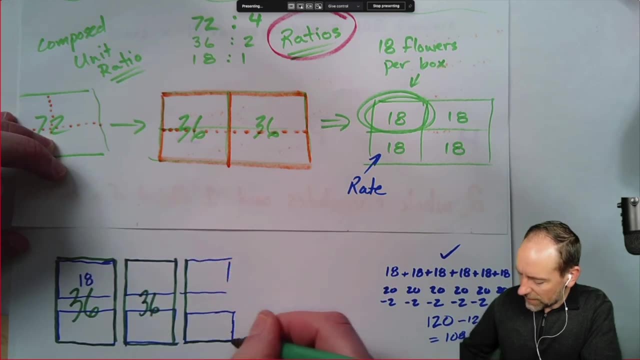 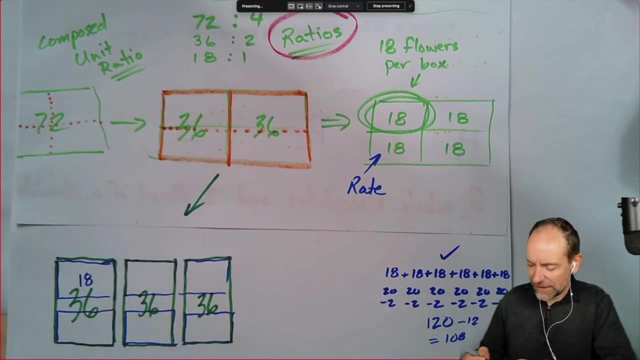 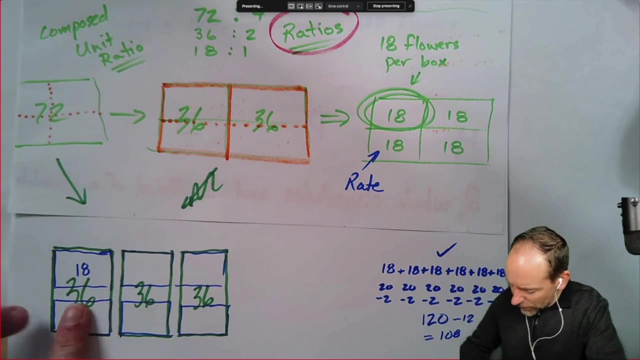 right, that means like this is 36 flowers and this is 36 flowers like all of it. now, if we think about this for a second or no, if i think about this for a second, four boxes is 72, like, And if I think about that and I go 36 plus 36,, hmm, 36 plus 36.. 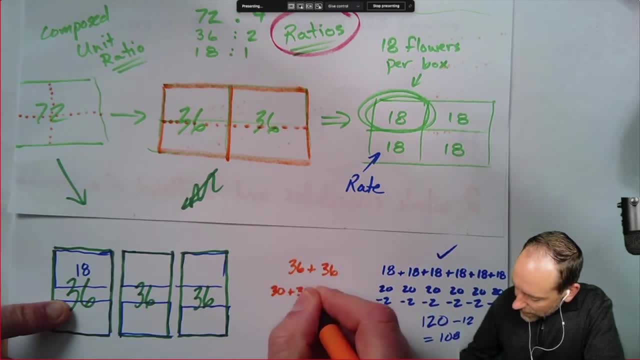 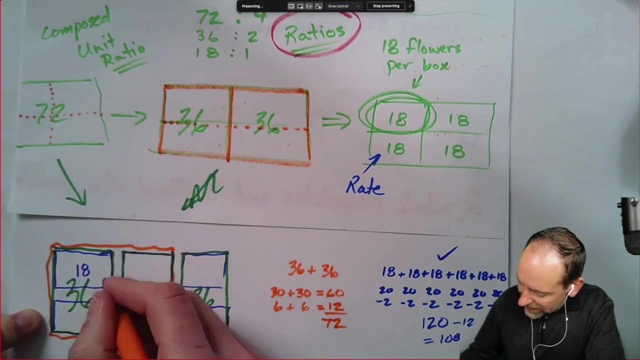 To me that's like 30 plus 30 and 6 plus 6.. So I've got 60 and 12 or 72.. Look at that. That 72 also works. So right here we have 72 in total. 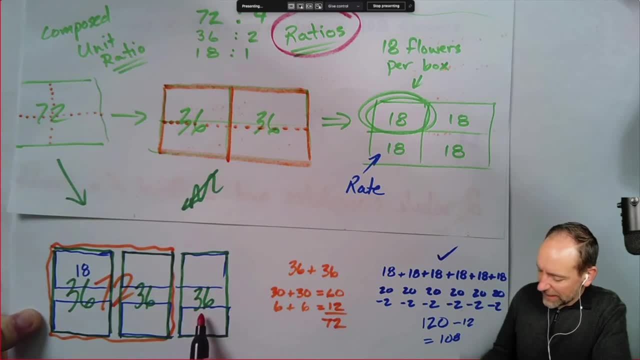 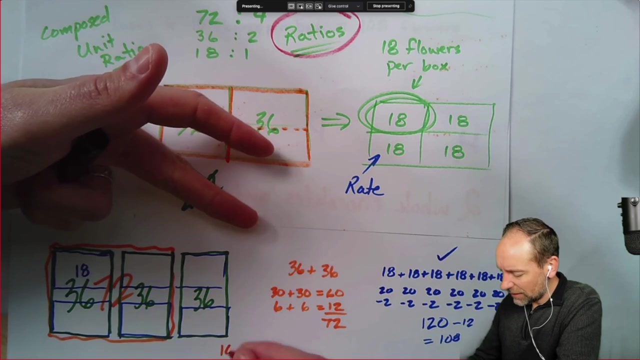 And then, if I just like add another 36, I'm good to go 72,, 82,, 92,, 102 plus another 6.. I think I feel good about 108 again. Holy smokes, Like we've got some interesting strategies going on here. 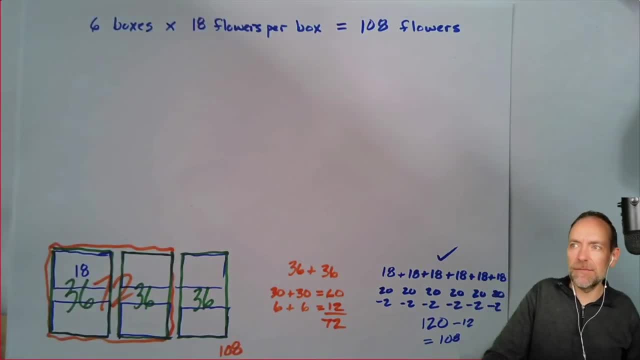 What do you say? I love it, I love that. That is awesome thinking, And I'm kind of looking at this and trying to think Of like how someone might do something like that. And you know, I mean I see it visually here. 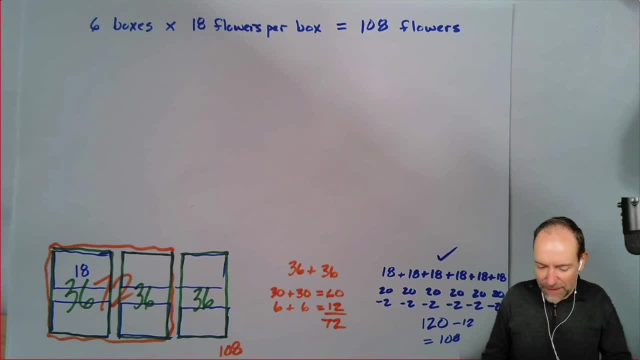 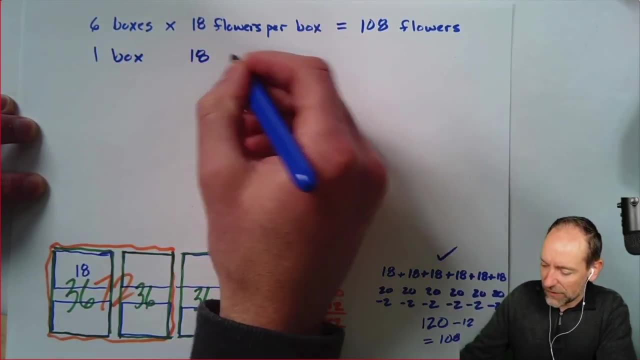 Like I'm even wondering about, like I'm like, well, maybe if I went back and I went, well, wait a second. I know what one box is. One box of 18 flowers is going to be 18.. And then I kind of see this like this doubling idea happening. 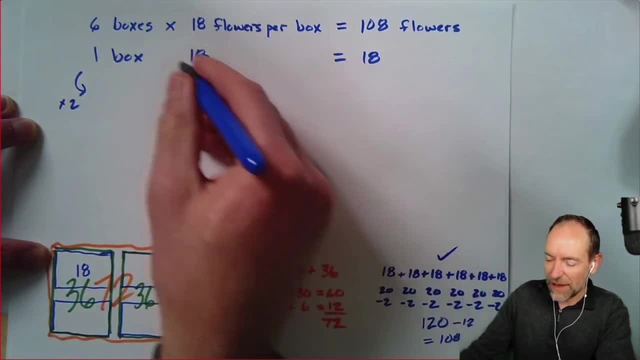 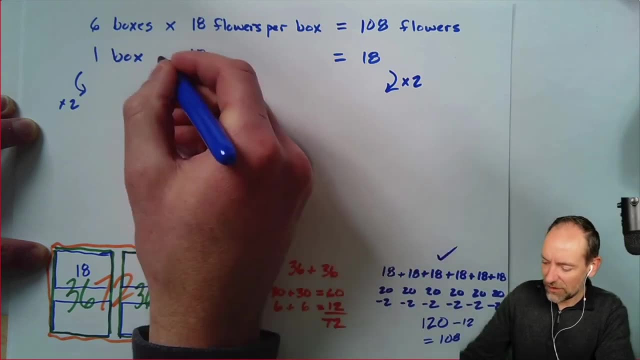 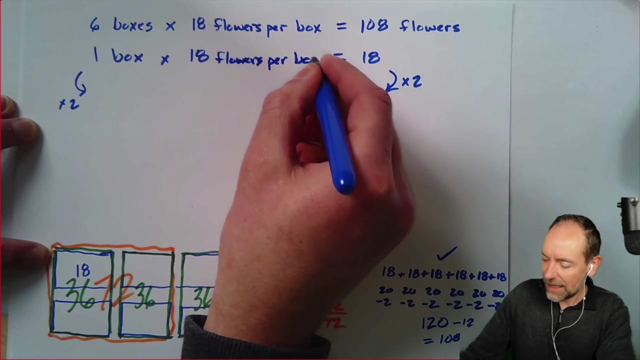 Like where I'm doubling this But I'm not doubling my flowers per box, I'm doubling my answer, Like it's happening in sort of a different place, Like my rate stays the same And it's like I can get there. It's like, well, one box now turns into two boxes. 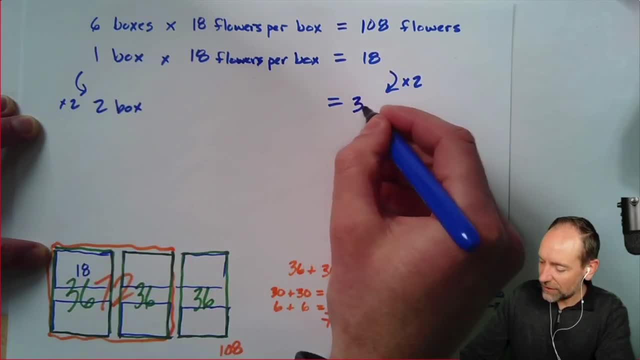 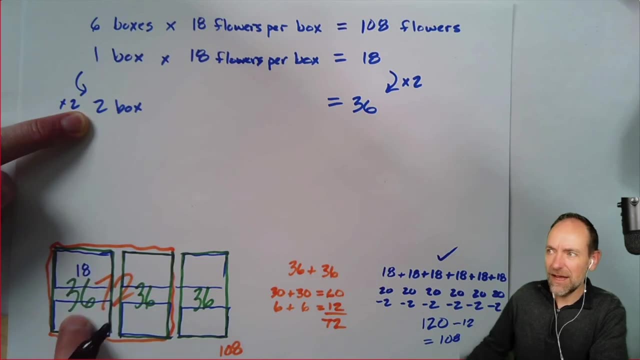 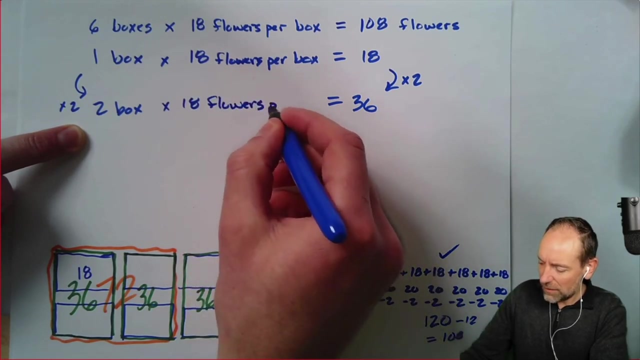 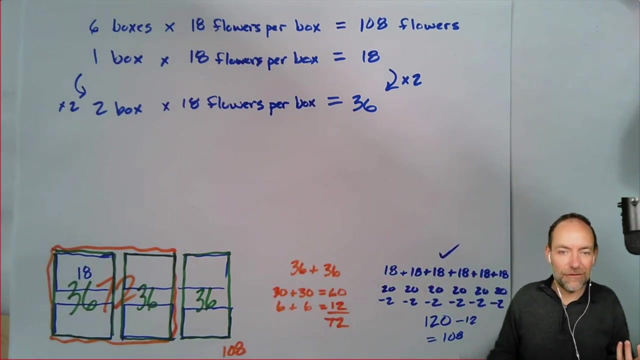 And 18 flowers turns into 36 flowers, which is consistent with what we're seeing here Right, Like when I doubled my 18.. Oh my gosh. There is so much interesting math that can be done here with multiplication, division and the idea, the idea of a ratio. 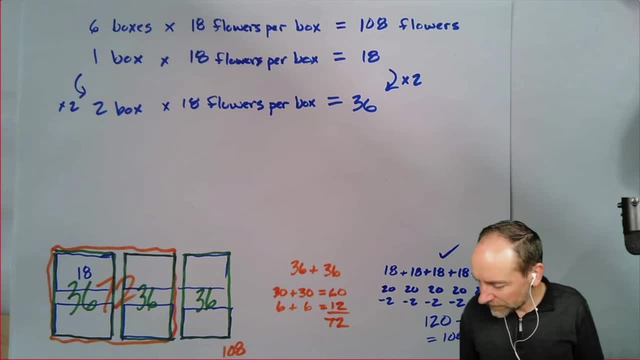 Right, Like that's pretty cool. I really like that Awesome, Awesome stuff. So any other information coming from the chat? And one of our friends who had a misconception earlier said on Monday I asked if it was 108.. We must have missed that. R is. 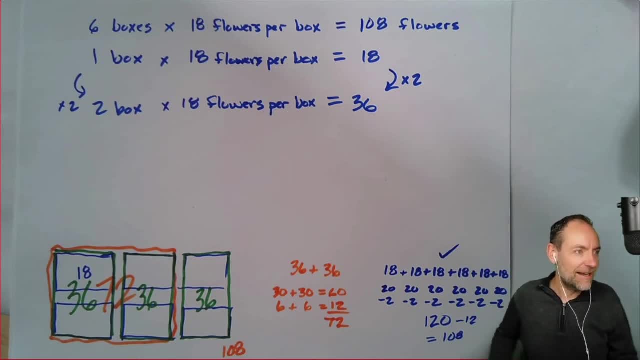 Yeah, And actually I see it now when I go back in the chat. I totally missed it, But awesome stuff And it's almost like you rethought your strategy or maybe didn't get confident with that strategy. So remember, go back and prove it to yourself. 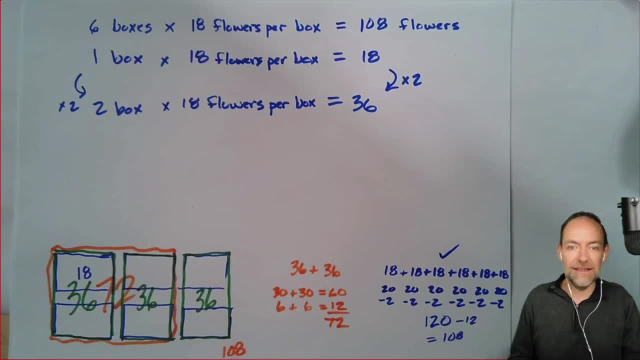 That's kind of like the main message from every math lesson that we've done is really it doesn't matter if you got the right answer or not. If you're not feeling good about the answer, then it doesn't really matter, Because it could be right. 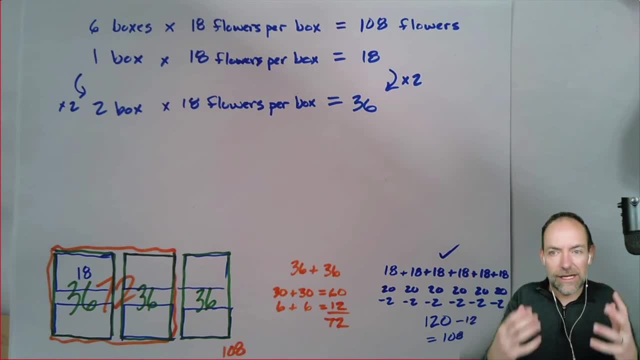 It could be wrong. It's just a gamble, Right? So let's make sure that we're really confident. you convince yourself there. All right, miss, What do you say? What time is it? I'm looking? Oh my goodness gracious. 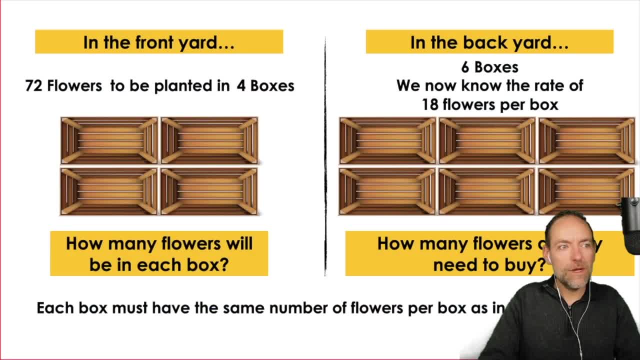 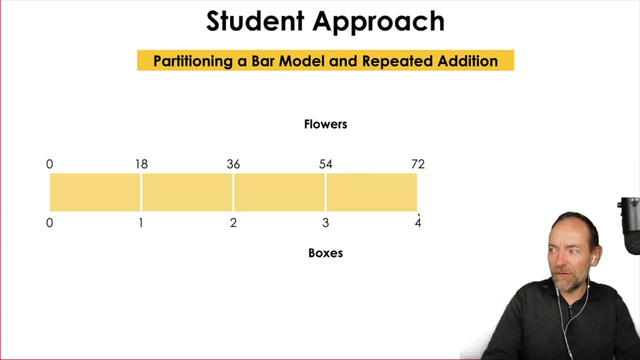 Where does the time go? I love it. I love it. We have so many, so many different strategies that we saw or that we used. If we go back and we sort of like give you another visual of you know where what we did with our 72 flowers and flowers. 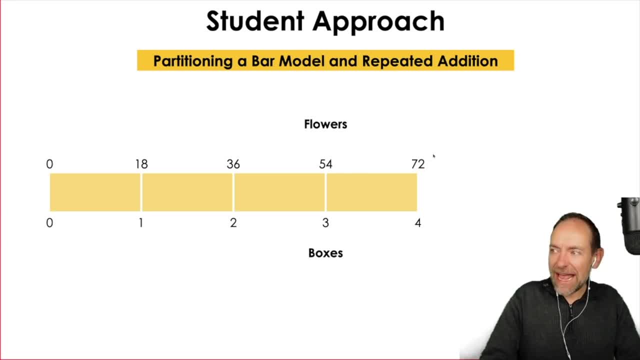 You can sort of see this, this, like if I half it and then I half it again. you can sort of see that idea coming to life here. And if we want to actually go and figure out how many were in, what did? we have six boxes. 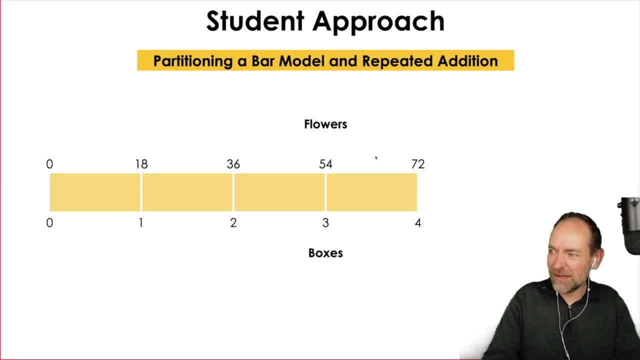 You can kind of see this idea that, hey, we could have started at four boxes and maybe just like added a box and 18 flowers and then added one again, Like that's a strategy that totally works, Totally love it And something. 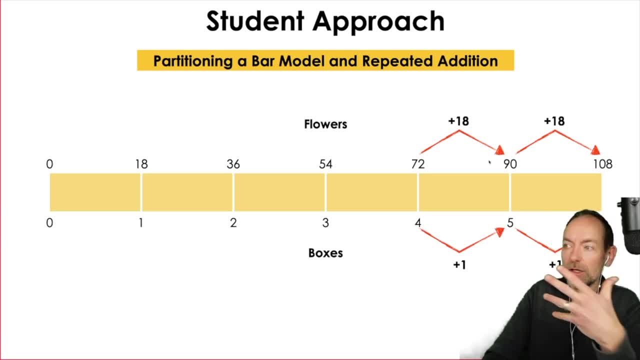 I'm also seeing here that I didn't think of before. This is the cool part about these strategies, right Is like you can see it different ways The more. the more you think about it, you see it in more flexible ways. But I see, when I add it twice, it's like I've added it once. 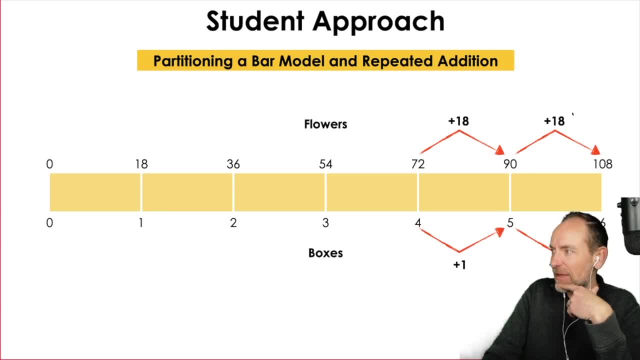 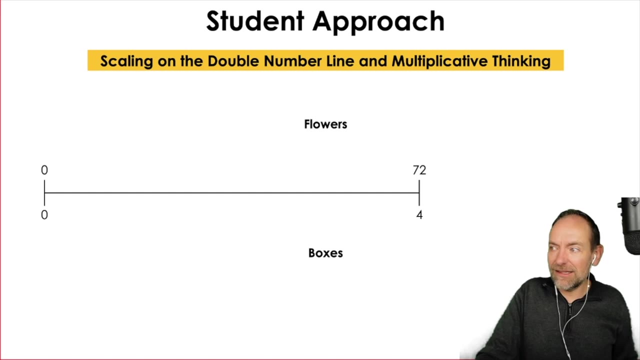 I've added it twice. It's like that is the same as that. So it's like adding it twice is the same as adding 36 flowers and two boxes. So I can actually use some of this information to help me as well. And again, one way is not better than the other, right? 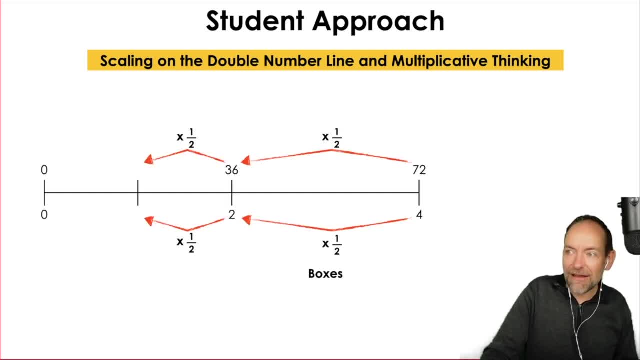 Like some people might have, like looked at this And again you see this like having idea going on on a, on a bar model, Right, And that really you know that might have been a strategy that you used And then, when you wanted to get to six boxes, maybe you just multiplied by six boxes, straight up. 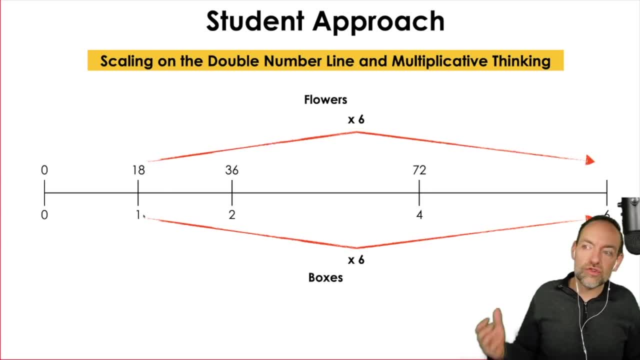 Like maybe you're really good with your 18s, or you have a strategy, Like maybe you went- you know what I want six groups of 10 flowers And six groups of eight flowers- And maybe that was a strategy that worked for you in order to get you all the way to your 108.. 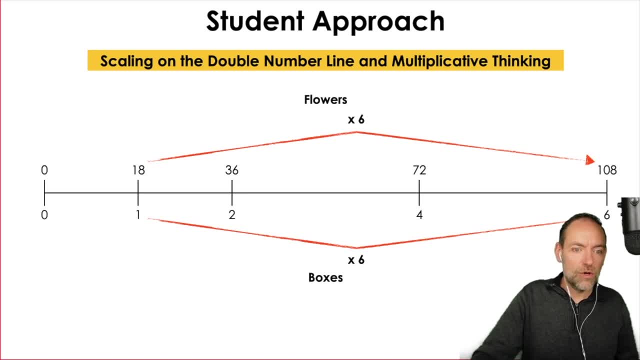 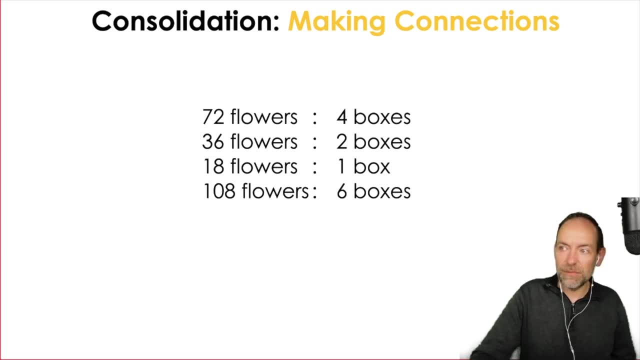 Like, totally up to you. There's lots and lots of really cool strategies that you could have used here in order to you know, to get to your answers. But, at the end of the day, what we're really working with is this idea of a composed unit ratio. 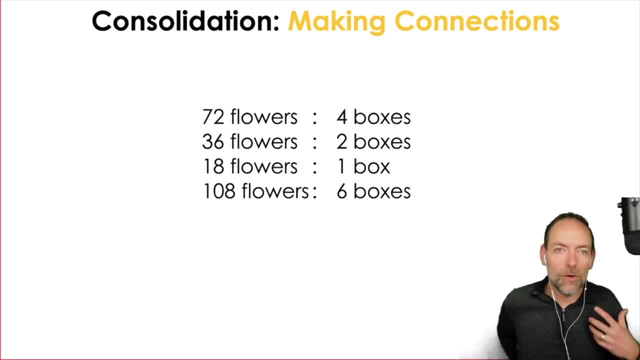 And that's sort of the big question. That, Or the big takeaway that we hope that you you have, is that all these ratios are equivalent and that I can use them and I can think of them as division and multiplication sentences. But I just have to be very clear on what it is that I have and what it is that I'm looking to find. 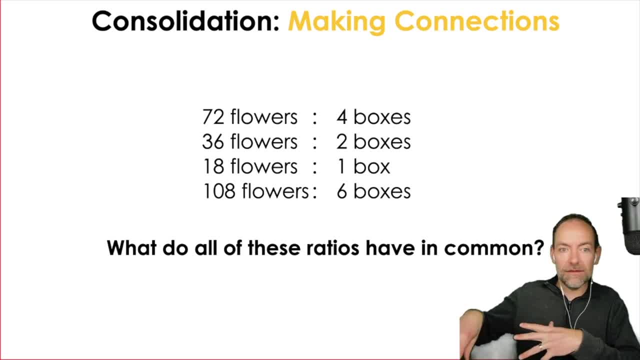 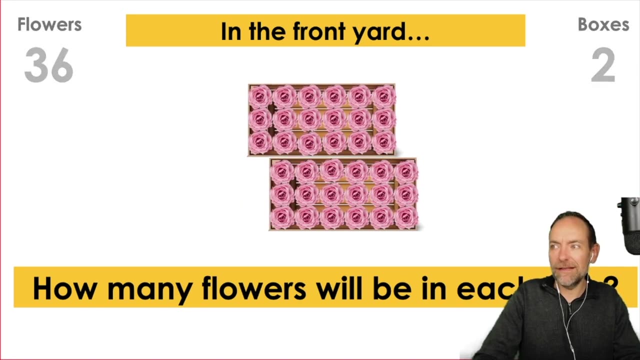 So think about the scenario: Don't strip away the units, like don't strip away flowers and boxes. Use these ideas in order to help make it easy and intuitive for you. Totally, totally, like looking at that and going like: oh, like, there they are, like nothing changed about the boxes, right? 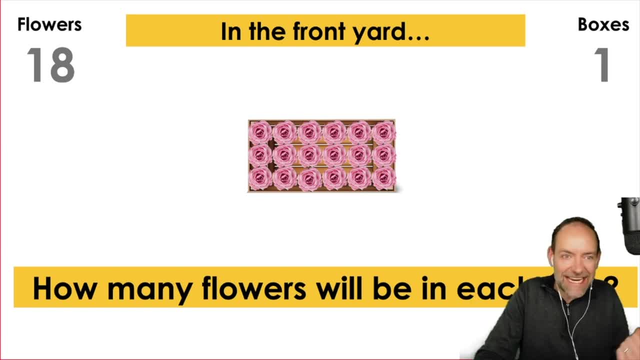 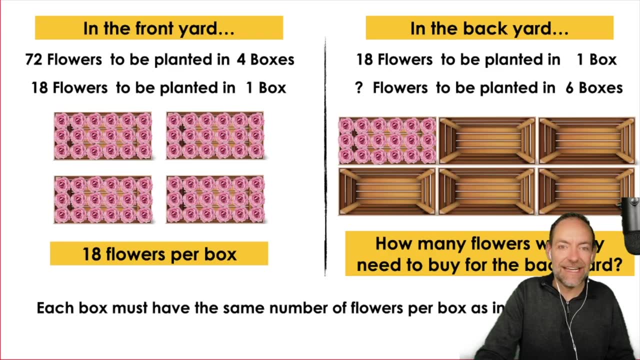 Like we just move them around, But the 18 stay, that rate stayed the same, And that is really, really important. And then when you start to see you know our backyard- and we start to see it's like, oh, like all we did was we just like made copies of what we already knew. 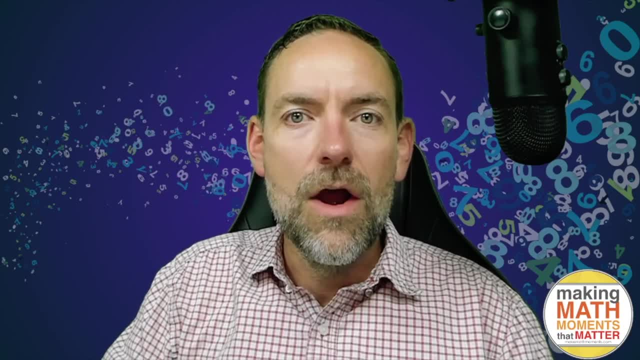 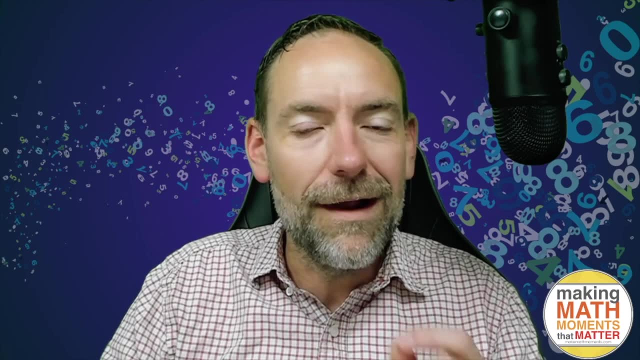 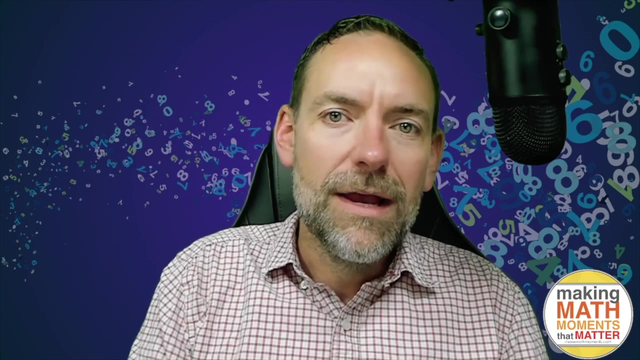 And here we are, Fantastic. Well, there you have it. Math moment makers. We are now finished that planting flowers day, one of that particular problem based unit, And I hope, if you haven't checked out the previous two videos, I hope you do, because we start off with sort of getting students started with a, with a number talk, with a math talk. 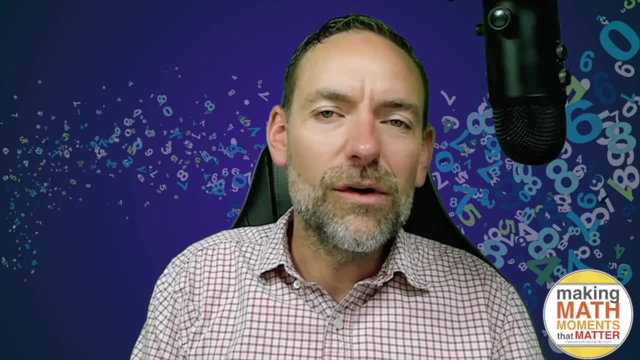 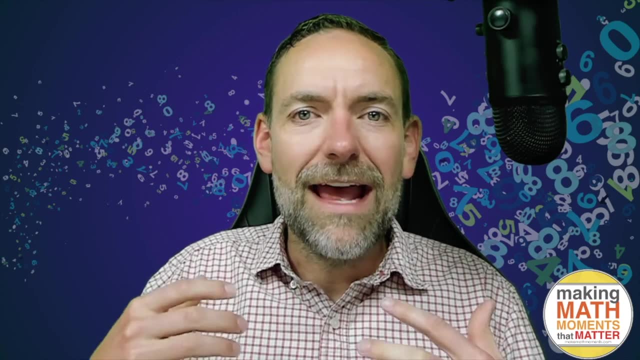 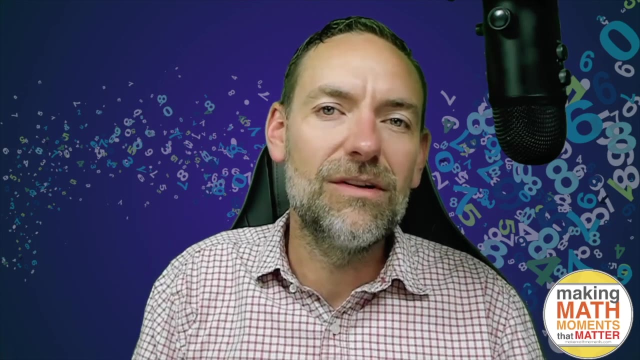 And then we extend this idea further in order to sort of emerge, through multiplication and division, in particular partitive division, Okay, from the tool. So See how we figure that out. Oh yeah, So we start off with a multiplication and division. 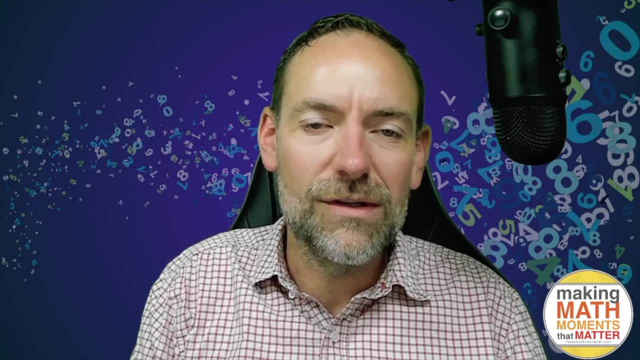 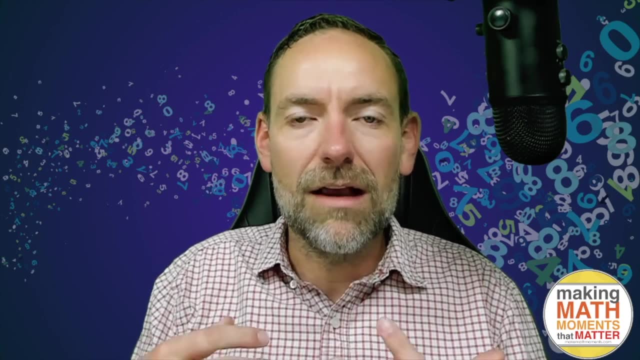 And again, for us It's a really weird concept, this set of equations which don't you don't get rzeczywiście, neither Get multiplication and division Get multiplication because we haven't done that much either. Now, The fine art of it is not actually sort of a key point, which is not really the key point, but we have to actually be able to take that into account. 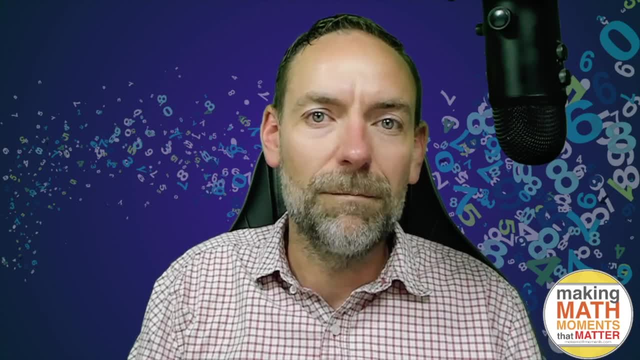 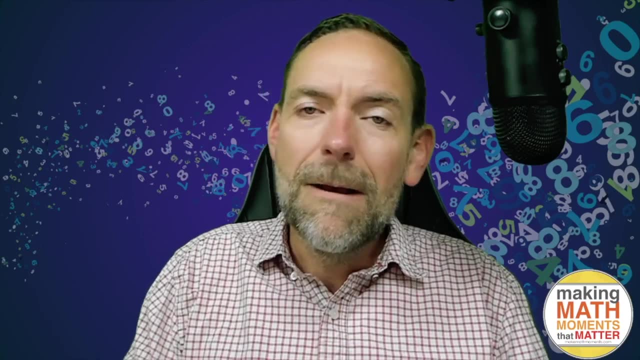 And again I love this metaphor: The high price is the small price. inematology and the into how that helps us realize a composed unit ratio means we're not promoting the use of calculators in these particular lessons. now, when we get to purposeful practice, maybe there's a role for a calculator there. but again, we want to encourage. 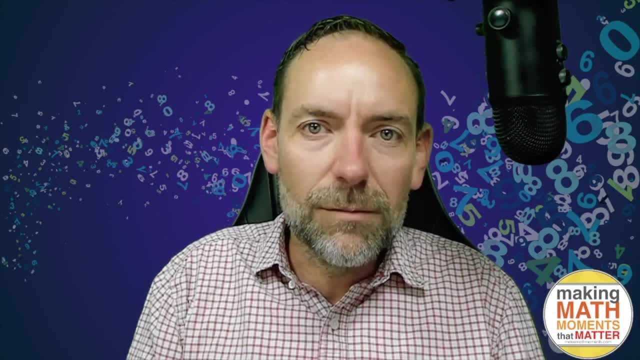 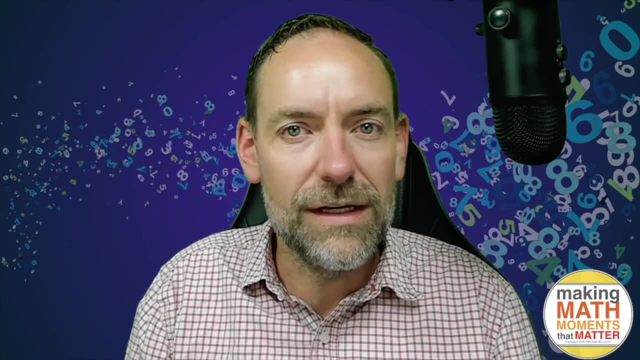 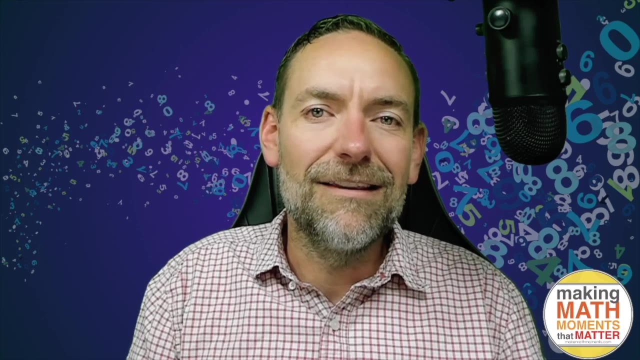 students to model their thinking. we want them to become flexible and fluent with multiplication, division so that when we get into the trenches with ratios, rates and proportional reasoning that students feel comfortable, they have a conceptual bedrock to stand on and they feel confident in their math classroom. now some of you might be wondering: where can you go in order to 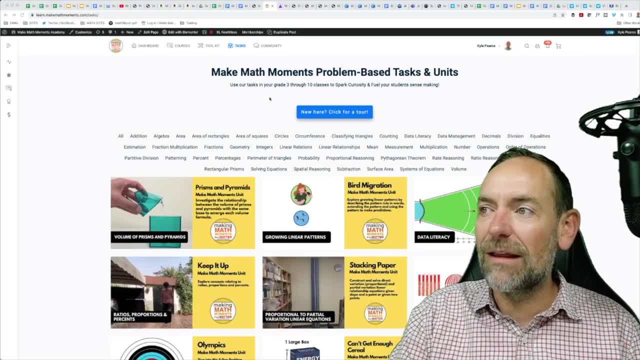 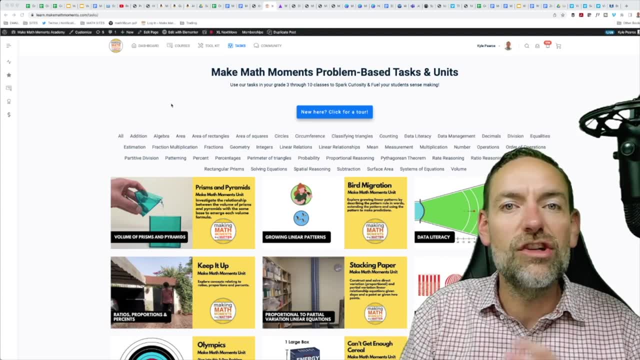 find this particular problem-based unit well. you can head over to the make math moments website, makemathmomentscom, and we have a tasks button there. or you could go to makemathmomentscom forward slash tasks. that will bring you to our tasks page now, right now, these- uh, it looks. 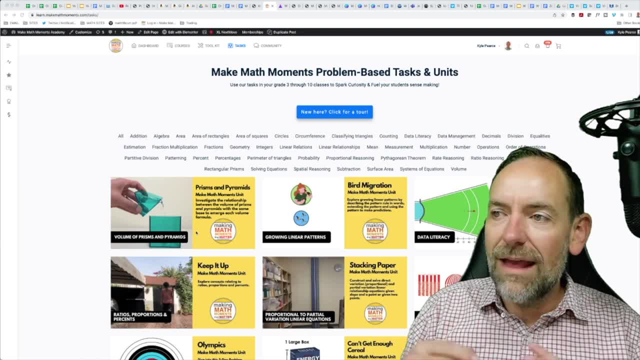 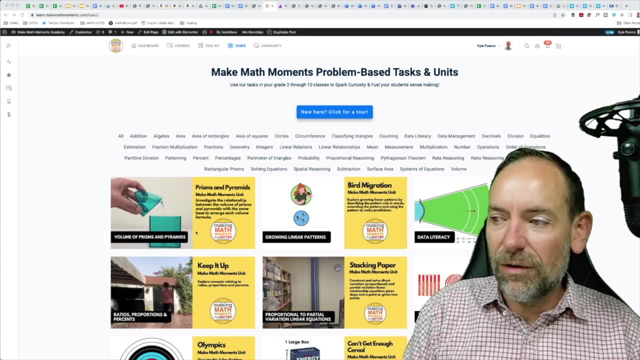 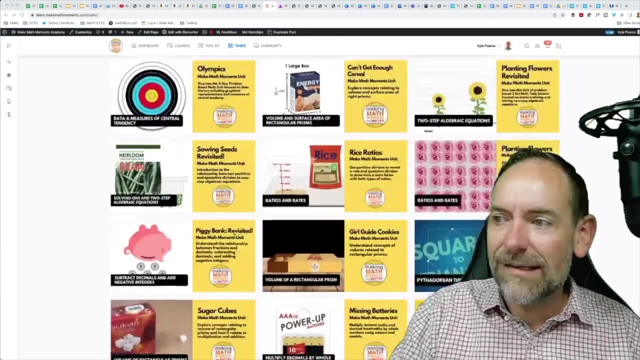 fairly, i'm gonna say un or disorganized, and that is because right now we are in the process of getting a continuum-based organizer ready to go. our web developer is currently working on that right now, but in the meantime you can search by topic and for us we were looking and working with our planting flowers. 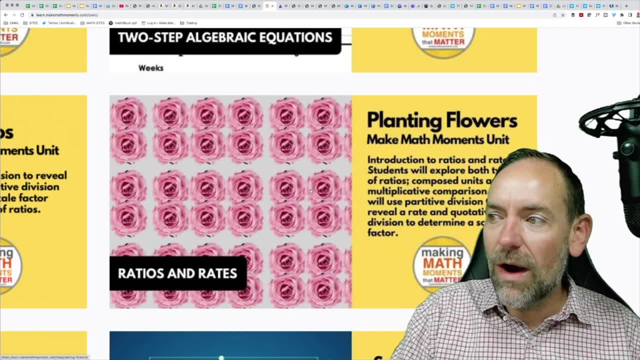 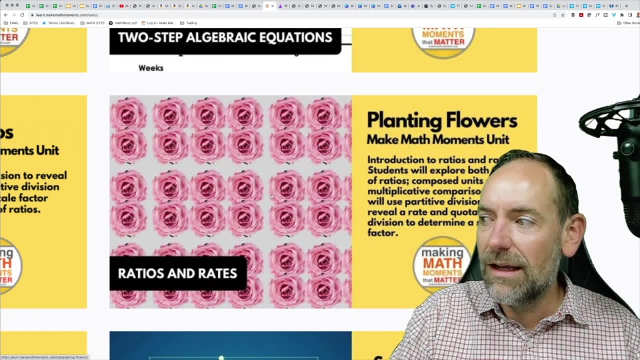 unit right here on ratios and rates. so again, while this idea is all about ratios and rates, really it's about multiplication and division and how they're intrinsically related, and this can be a really great opportunity for you to dig into classifying your math classroom and how you can do that. and i'll see you in the next video. 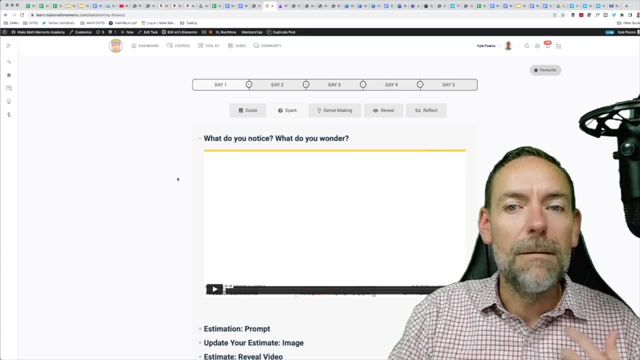 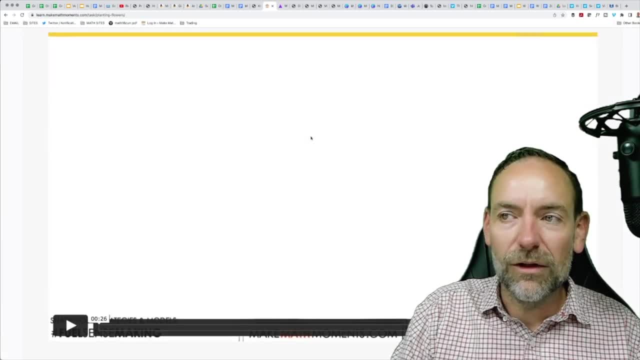 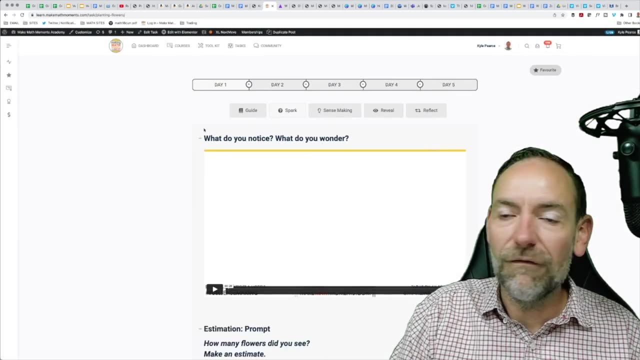 context, rich problems with your students that promote the emergence of big ideas, strategies and models, and really it's all for you right here to run from the web including all of our video clips and our prompts- all kinds of wonderful, wonderful learning to be had. it is a five-day unit and all. 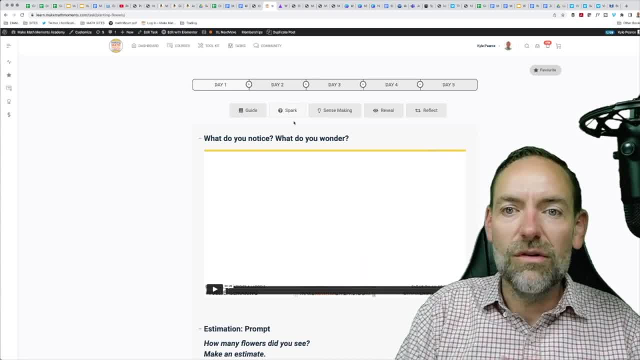 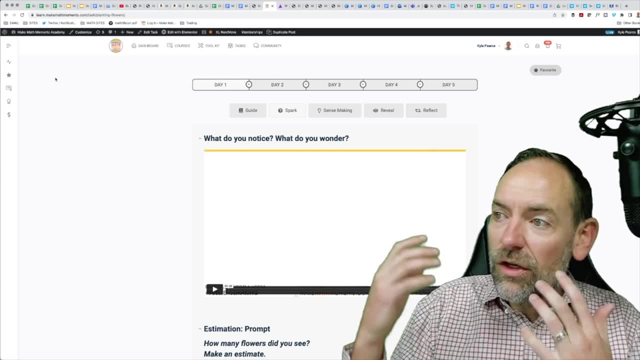 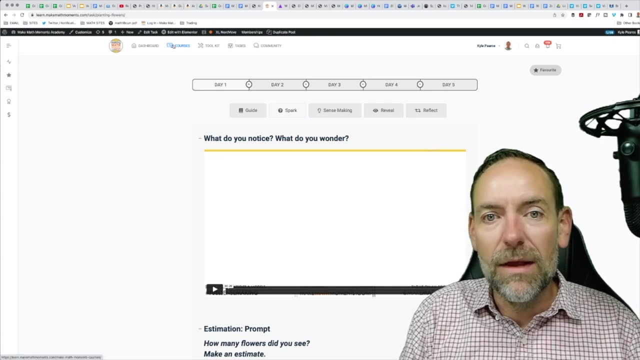 of day one is open for you to use in your classroom as you see fit, and then portions of the other days are there as well, of course. if you want to join the academy, you will gain access to all the problem-based units, as well as all of our courses to help up your game. 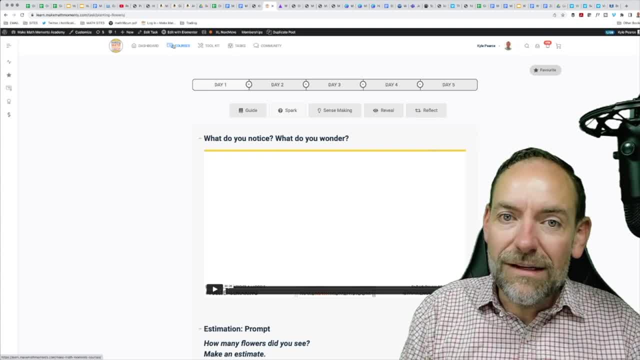 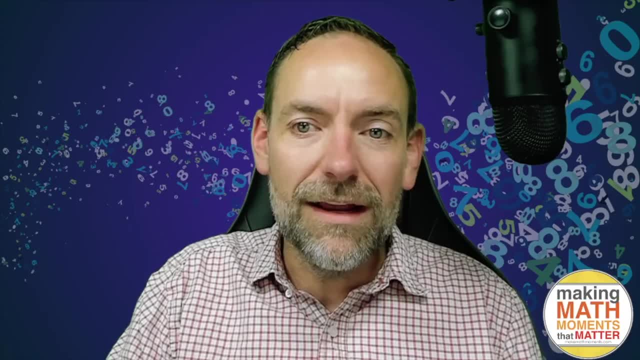 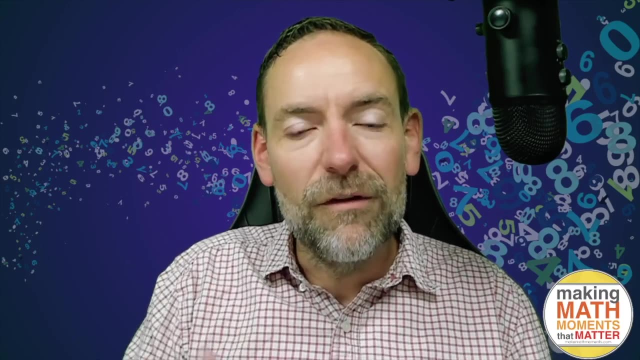 in your classroom right now. if you haven't done so yet, do us a favor: hit the subscribe button, hit that notification bell and like this video. it'd be great if we got some of you to share a comment. what did you learn here? what are you going to implement tomorrow, maybe a month from now, and